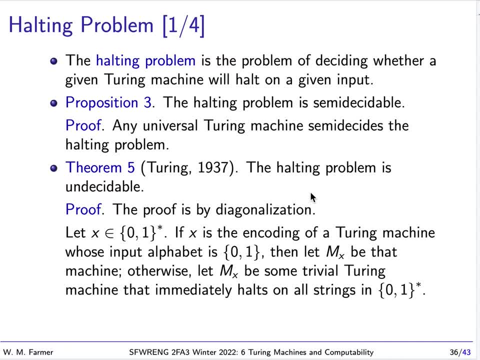 input to the input for m and be able to determine in all cases whether that Turing machine will halt on x or not. So the halting problem is undecidable and we're going to show this by diagonalization. This proof is similar to the proof that we use to show that there are uncountable sets. that's due to. 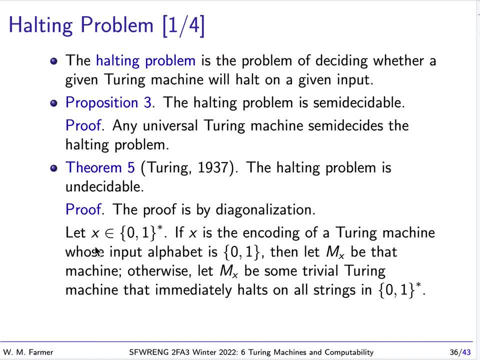 Cantor. Okay, so let x be a string of zeros and ones, and if x is a encoding of a Turing machine whose input is zeros and ones, let then let m of x be that machine. So we're going to restrict our attention to Turing machines whose input 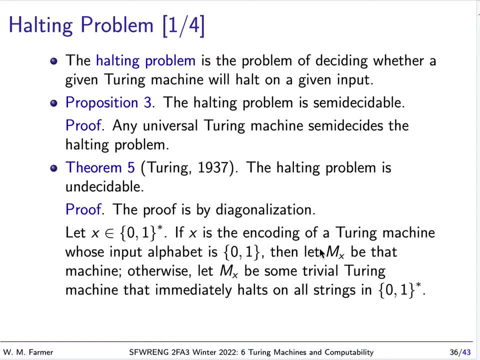 alphabet is zero and one, and M will be the machine that corresponds to the encoding of this Turing machine. Now, if x is not an encoding of a Turing machine, we're going to let x be some trivial Turing machine. that is sort of always in our complications. 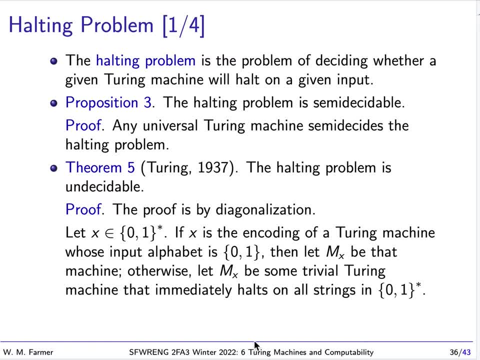 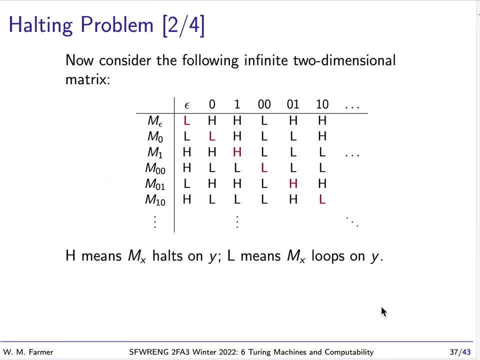 that immediately halts on all strings over the alphabet 0 and 1.. So for every x, every string of 0s and 1s, mx will be a real Turing machine. Now consider the following infinite two-dimensional matrix: So here we have all our Turing machines. 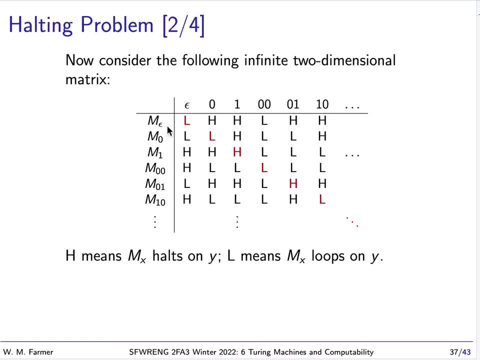 These Turing machines correspond to strings of 0s and 1s. so we have the simplest string, the empty string, the string of just 0,, the string of 1,, the string of 0,, 0, and so forth. 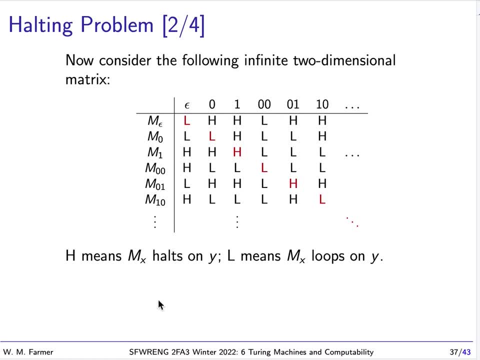 So down this column we have all possible Turing machines, and on this row we have all possible inputs, and so this matrix will tell us what happens with every Turing machine on every possible input, And h means that the Turing machine halts on the input and l means the Turing machine. 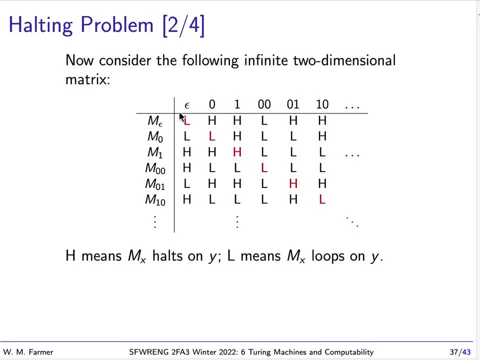 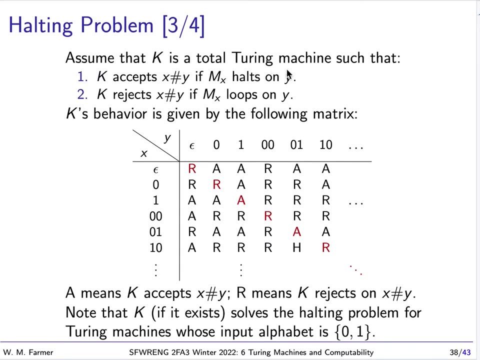 loops on the input. So there exists some such infinite two-dimensional matrix. So now let's assume that k is a total Turing machine that has the following property: So k accepts This string x sharp y if m of x halts in y, and it rejects x sharp y if m of x loops. 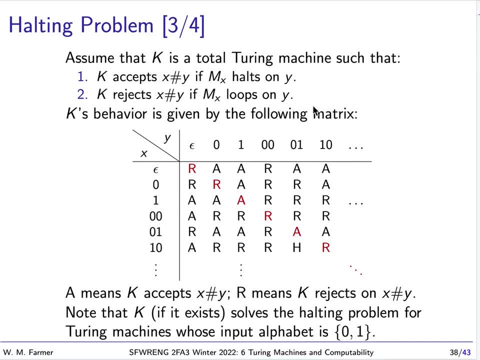 in y. So k's behavior then is going to be given by the following matrix: If x is a code for a Turing machine and if y is the input, And then a means that x accepts the string and r means, I should say, k accepts the string. 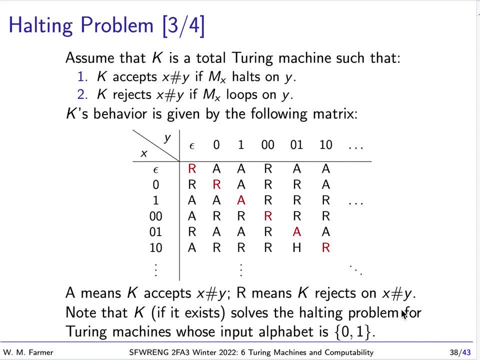 and r means x rejects the string. And the thing to note here is, if there actually were such a total Turing machine k, this k would solve the halting problem for all Turing machines whose input alphabet is 0 and 1.. So remember, we're restricting ourselves to just Turing machines whose input alphabet. 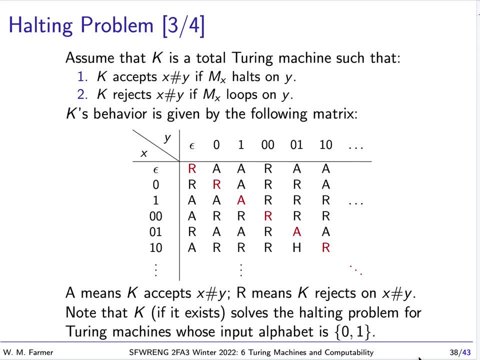 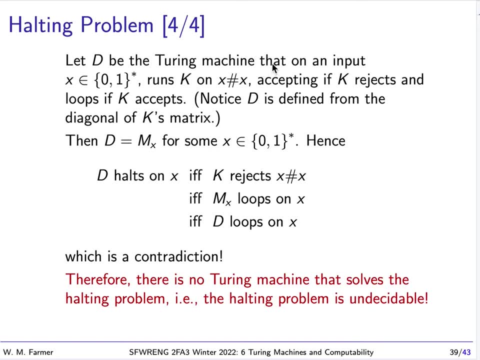 is 0 and 1.. So we're going to assume there is such a k. Now let d be the Turing machine that on input x runs k, on x sharp k and it accepts if k rejects and it loops if k accepts. 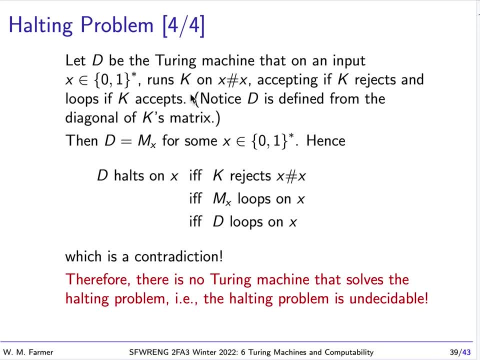 Now this makes sense Because k rejects k is a total- Remember, k is a total Turing machine, And so d is going to be defined by the diagonal of k's matrix. So when k accepts- well, I should say when k rejects- d is going to accept. 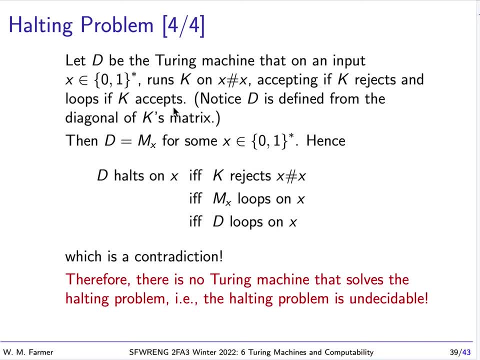 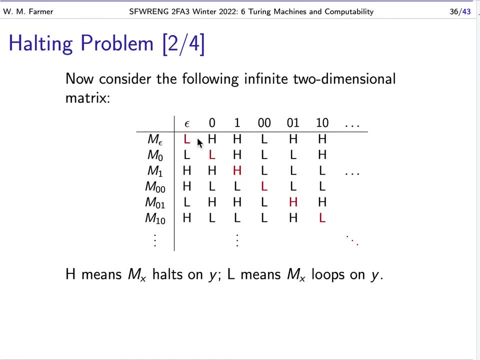 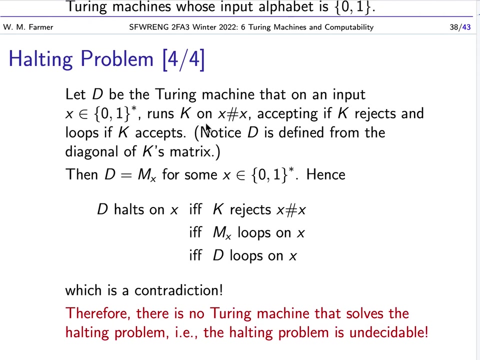 And it's going to loop when k accepts. So if we go back up here, what d is going to do is it's going to, it's going to. let's go back. go back to this a moment. So k is going to accept if k rejects and it's going to loop if k accepts. 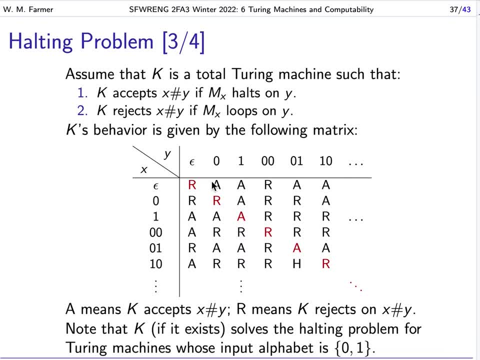 So d is going to accept if k rejects and it's going to loop. if k accepts, k will meaning with k negative k it's going to so when? so when along here, when k accepts, d is going to reject and when k rejects, d is going to loop. let's see, did i get that right? 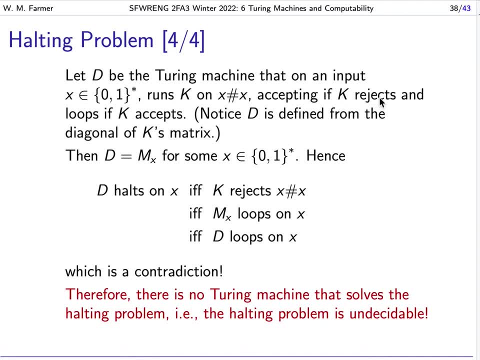 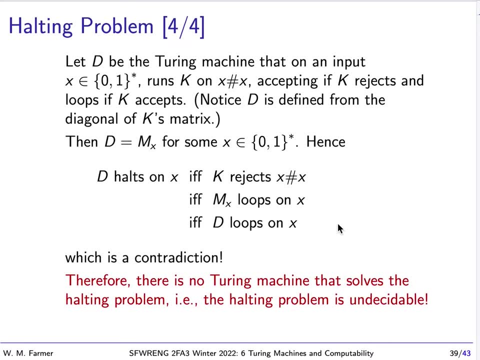 no, when. when k rejects d accepts and k accepts d loops. okay, so now, um, what we do is we? we know that d is a turing machine whose input alphabet is zero one, so it's going to equal mk for some x, some string x, and now d halts an x. 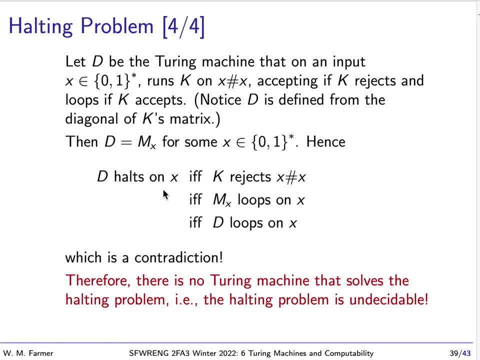 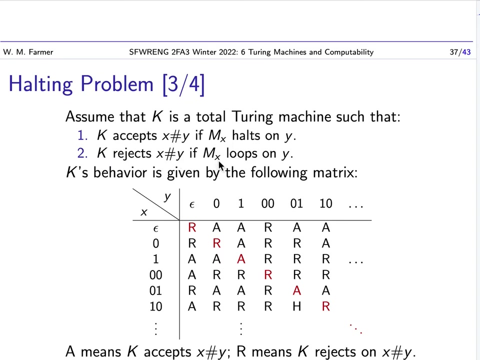 so well, d halts an x means that k rejects, so that means k rejects this. and if k rejects this, this means that if we go back up what k does, k rejects this string if mx loops in y. so this means if k rejects x and y. 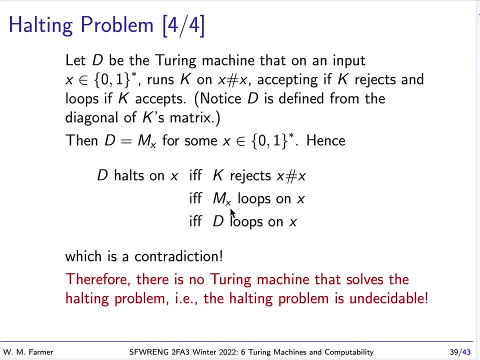 well, d halts an x means that k rejects this string if mx loops in y. so this means, if k rejects x, that means mx loops on x and mx is d, so this means d loops in x. so we've just shown that d halts an x. 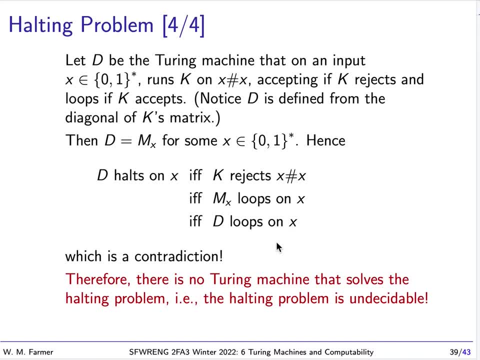 if, and only if, d loops an x, which is an impossibility. this is a contradiction. so therefore, there is no turing machine that solves the halting problem. so, specifically what we've shown, there's no turing machine that solves a halting problem for turing machines with alphabet. 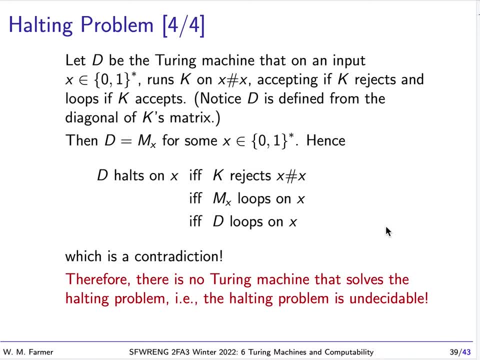 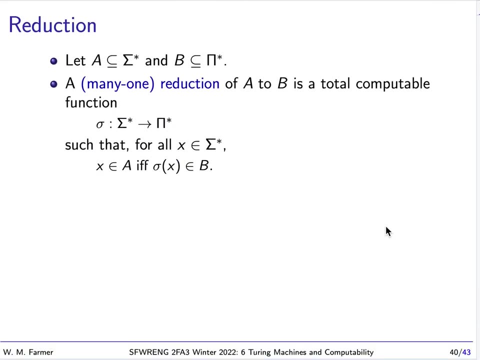 zero and one. so this is essentially what turing showed, and this is a one of the many important proofs in the theory of computation that uses a diagonalization argument. okay, so now we're going to look at the notion of reduction. so with reducing, we have a set a and a set b, the set d and the set e. well, if you Python lose one, I'll have to do a column. on a indicator scale, we'll prone to y, and so it's a long subscribers rather than 6, and let's try allows you to try and sum up to y, and so yours n and y is powers plus 5. y equals n, equals y plus 1, so those numbers are 0, then 2. 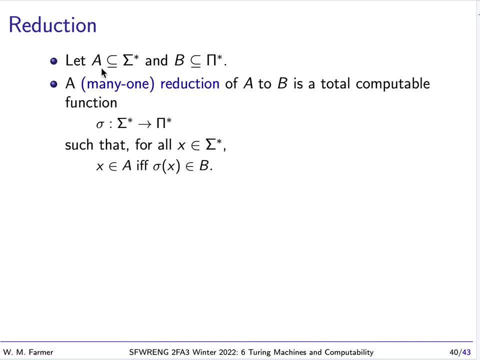 set a and a set b. the set a is over some alphabet sigma and the set b is over some alphabet pi. and we say we have a reduction which in sometimes we call a, many one reduction of a to b is going to be a total computable function from strings of sigma to strings of pi. 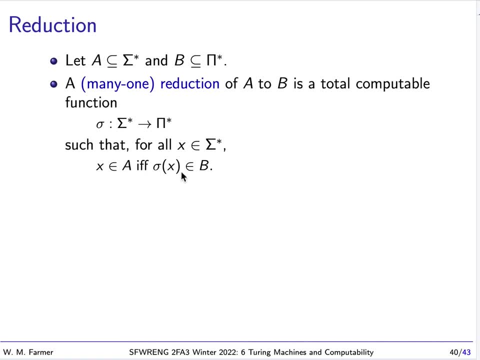 such that x is in a if, and only if, sigma applied to x is in b. so basically, this maps every member of a to a member of b and, and the important thing here is that this is a total computable function. okay, so so we will say: a is reducible to b, which 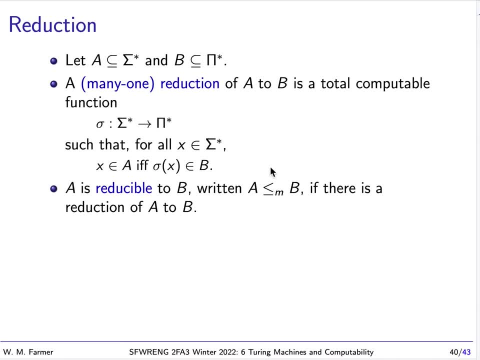 we will say a is reducible to b, which we will say a is reducible to b, which we write like this: a is less than or equal m and m means this is so. it's many to one, it's many one, because a string, several strings in a, can go to the same string in. 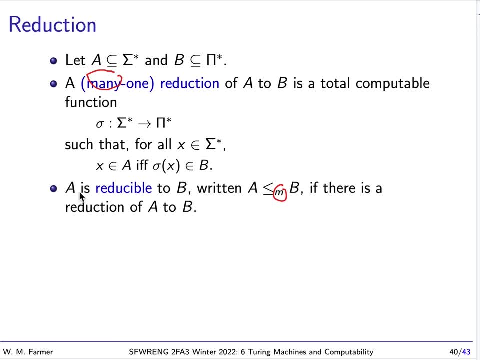 b if, if we want anyway, we'll say a is reducible to b. if there is a reduction of a to b, and now we have a proposition for which says: if a is reducible to b, then Then B is RE, implies A is RE. 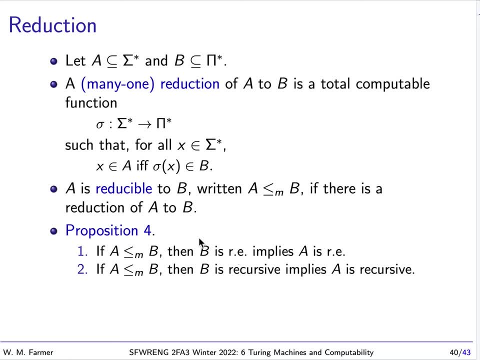 So how do we know this is true? So let's assume A is reducible to B and B is RE. So if B is RE, there's going to be some M that accepts B, Some M that accepts B, And so we can come up with now a machine that will accept A. How does this work? 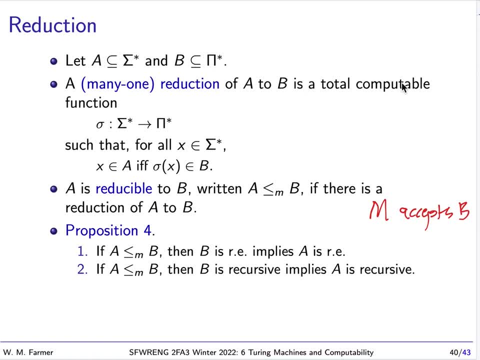 The machine will. since there is a total computable function, there will be some machine for this function. I'll call it n? sigma And what we do is we give n n sigma And it will compute sigma. Or I should say, we'll give n sigma x and it will compute sigma x. 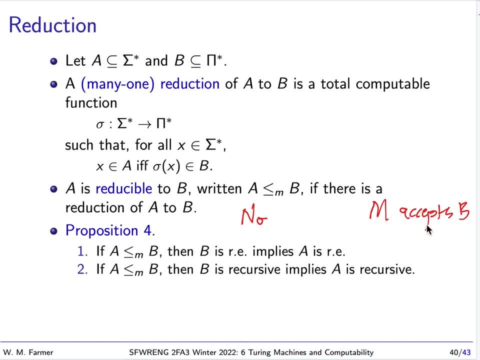 And then we'll give that sigma x to M and it will compute whether it accepts that, whether that sigma x is in B, And if it is in B, then we know by the construction of this total computable function that x is in A. Therefore we have a Turing machine that accepts A. So 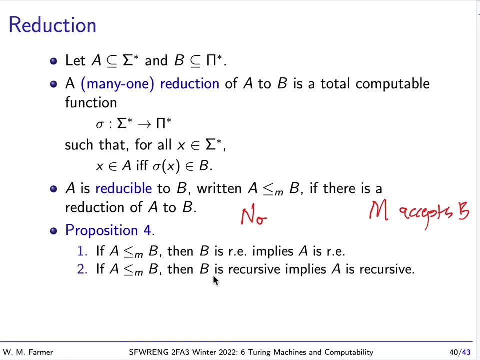 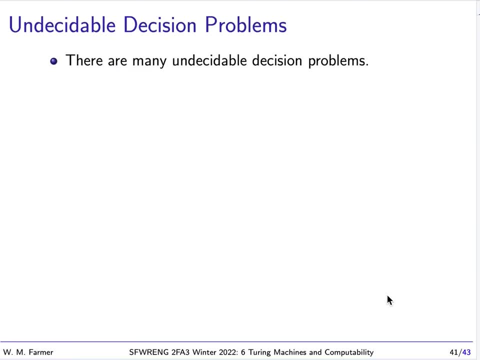 we know that sigma x is in B And the same basic argument shows that if B is recursive, that implies that A is recursive. Now there are many undecidable decision problems. They're not rare, They're quite common, And there's two techniques for showing that decision problems are undecidable. 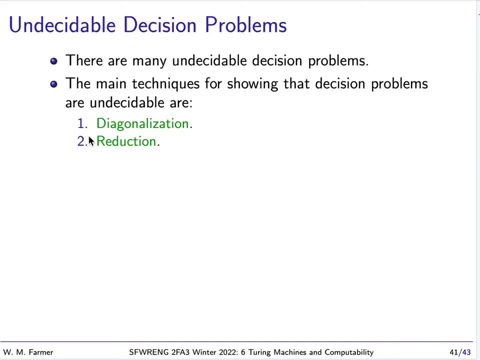 There is diagonalization and there's reduction. We've already seen how diagonalization works. We've shown that the halting process works. We've already seen how diagonalization works. We've shown that the halting process works. The decision problem is undecidable. 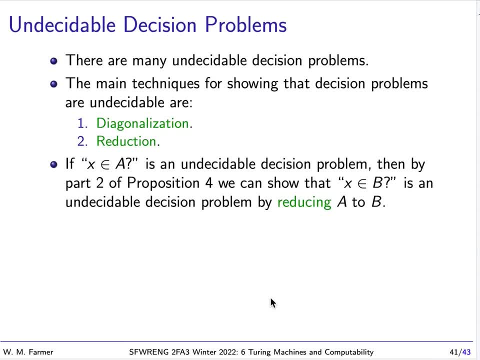 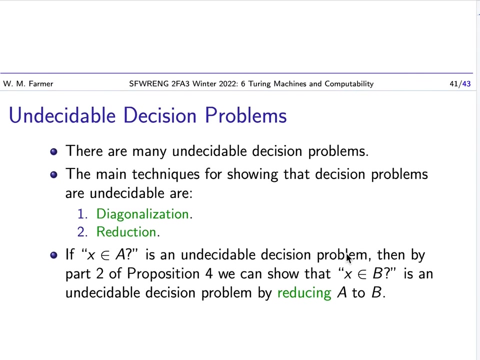 So if x is a member of A is an undecidable decision problem, then by part two of proposition four we can show that x is a member of B is an undecidable decision problem by reducing A to B. So basically the idea here is to reduce A to B. 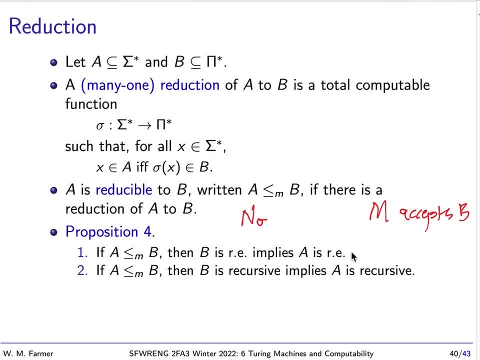 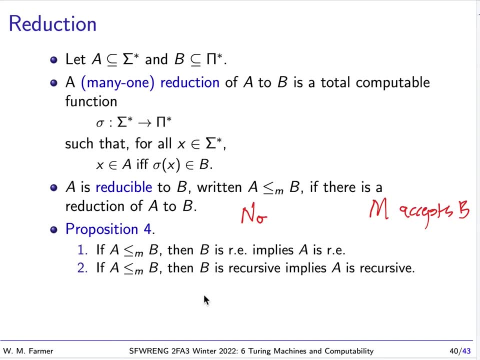 So if x is a member of A, then we can show that x is a member of B. is an undecidable decision problem, If we know. if so, we have this statement. the contrapositive says that A is not recursive implies B is not recursive. 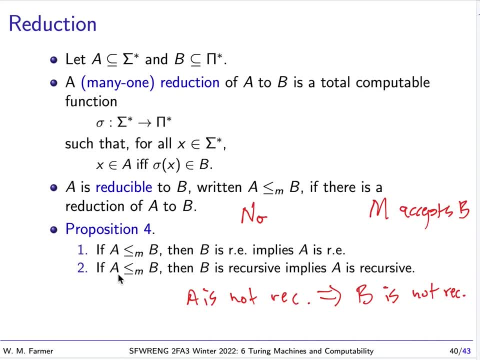 So we find an A that's undecidable, we reduce it to B and then, by this proposition, because A is undecidable, therefore it's not recursive, that means B is not recursive, therefore B is also undecidable. 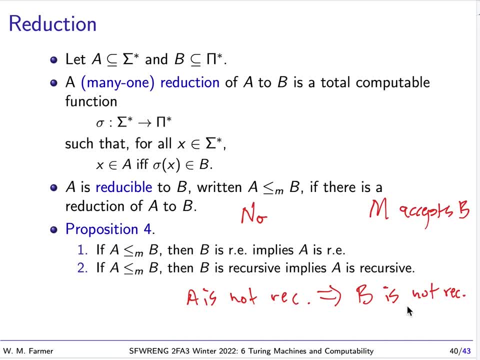 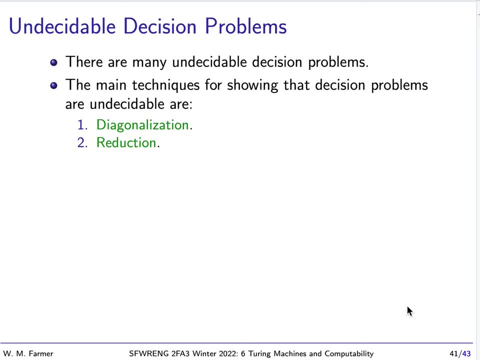 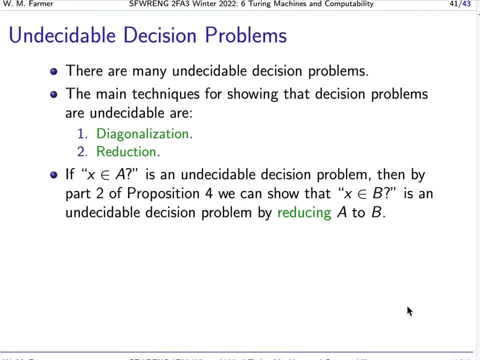 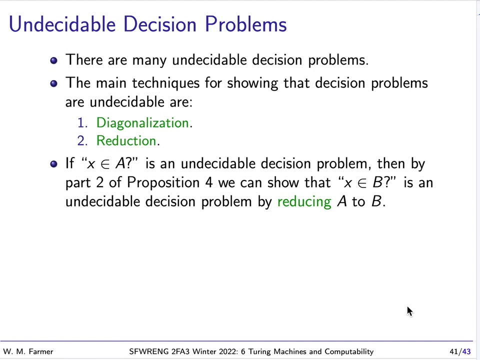 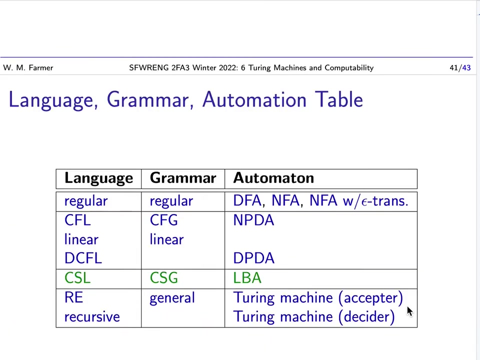 So by using reduction, we can show that other problems are undecidable by reducing, By reducing to those problems, problems we know are already undecidable. So to sum up, once we have some undecidable problems which we show by diagonalization, then we can use reduction to show that many, many other problems are also undecidable. 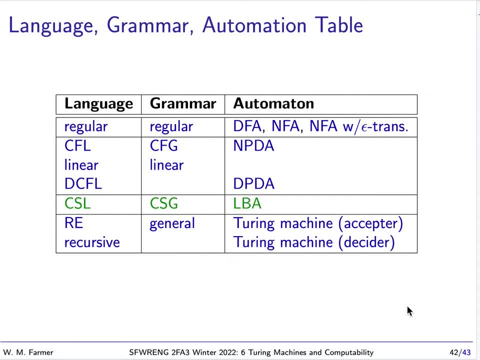 Okay, So this slide of all our lectures. it basically sums up what we've looked at for the latter part of the course And you've already seen this table. It's a table of languages, grammars and automata And we have four kinds of languages corresponding to the Chomsky hierarchy: regular, context-free and context-sensitive, and recursively enumerable. 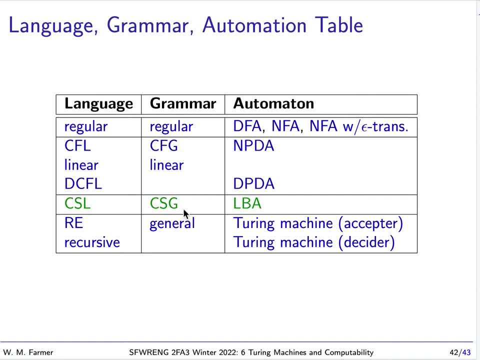 We have four kinds of grammars: regular grammars, context-free grammars, context-sensitive grammars and general grammars. And then we have various automata. For regular, we have DFAs, NFAs and NFAs with epsilon transitions. 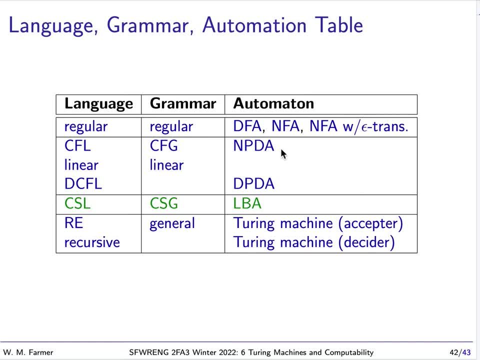 For context-free we have nondeterministic pushdown automata And for context-sensitive we have linear bounded automata And for RE we have Turing machines. Now the part in green deals with context-sensitive languages. We really haven't spent much time on these because they're not so important for computing as all the other languages are. 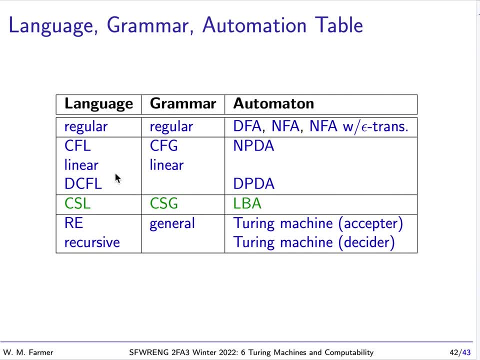 We've also noted some subdivisions. So some context-free languages are linear, Those are languages that are generated by linear grammars. And there's also another subgroup of languages: Deterministic context-free languages. Those are languages that are accepted by deterministic pushdown automata. 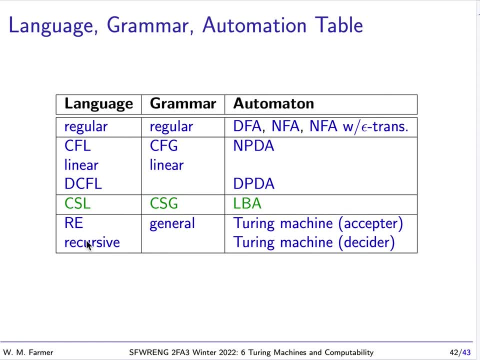 And another very important subset of languages, of recursively enumerable languages, are recursive languages. These are languages that are accepted by total Turing machines. Because they are accepted by total Turing machines, the Turing machine actually not only accepts the language, but it's a decider. 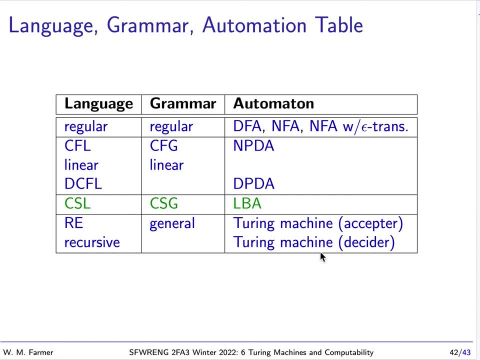 It can decide whether a given string is a member of that language or not. So this completes the lectures for software engineering 2FA3.. Thank you very much for your attention. Goodbye. 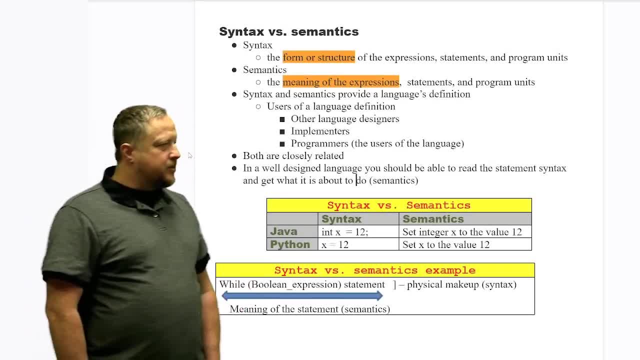 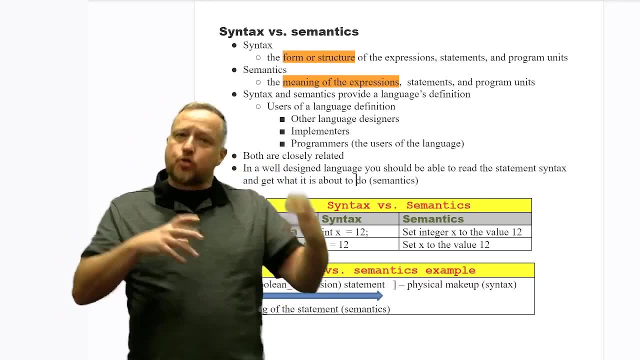 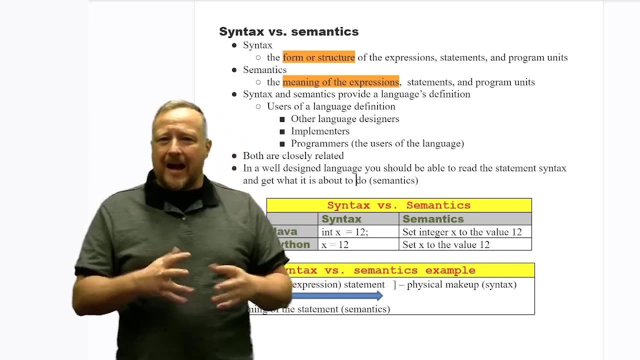 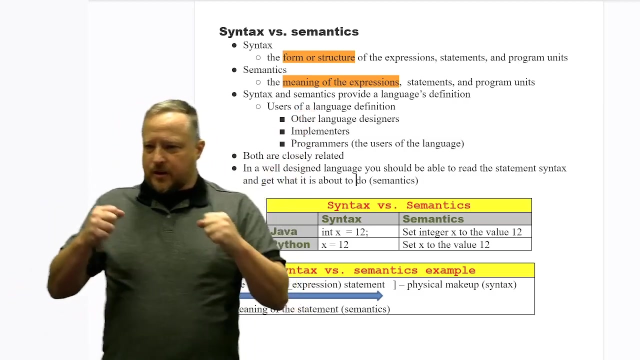 So what's the difference between syntax and semantics? Syntax is the physical layout of the structure for each one of the statements, expressions, loops, functions, calls, all that. It's the physical layout. The semantics is the meaning behind all of it, With the units. 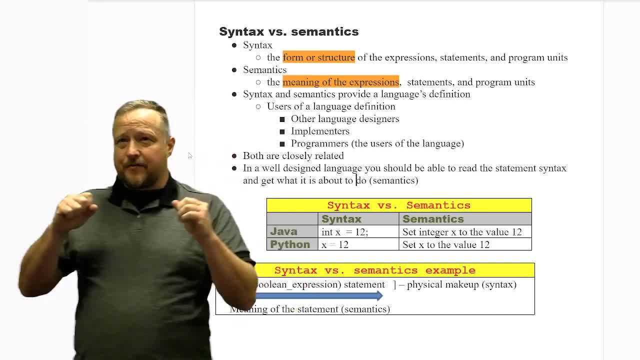 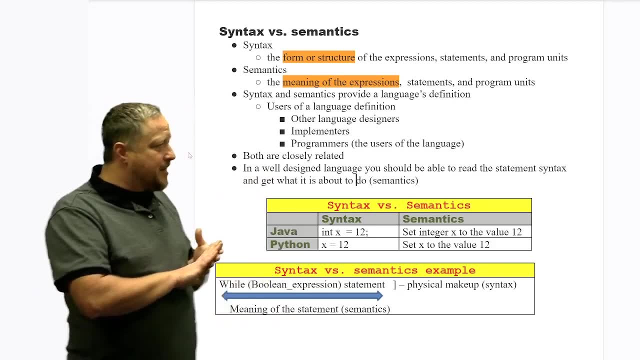 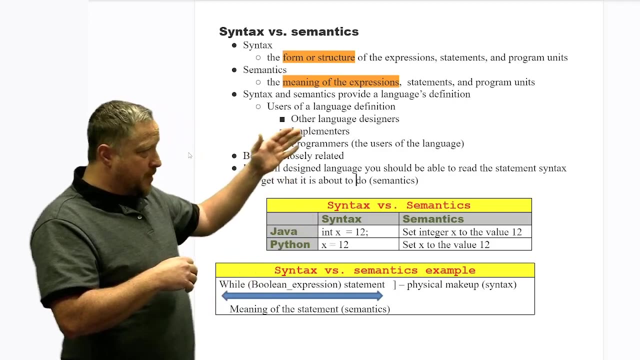 it doesn't have data structures, doesn't have declaration of data types. That's the meaning behind it. So both the syntax and semantics provide the language's definition, And the language definition is going to be used, maybe by implementers, by programmers and other language. 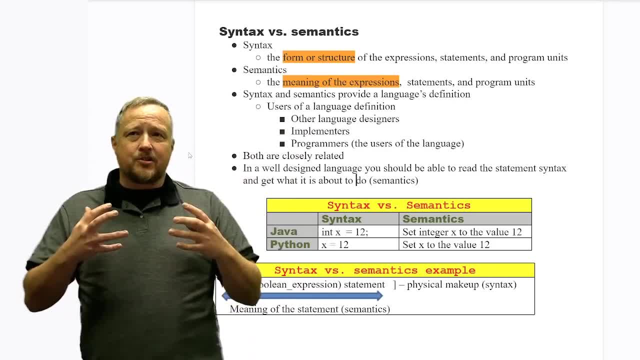 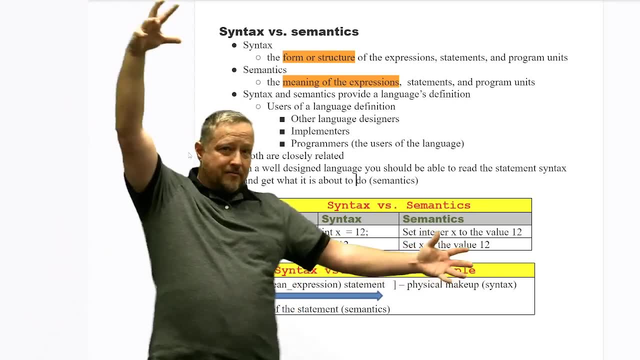 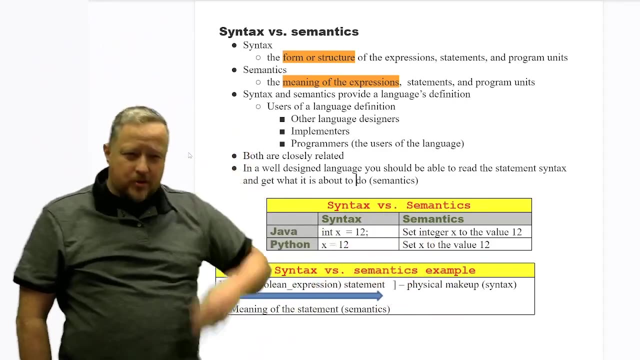 designers. They're going to try to make this as easy as possible. called also syntactic sugar Meaning you might be able to do it in really really a lot of statements in one language, But in the current language you can do it in one or two lines, So they're constantly thinking about that. 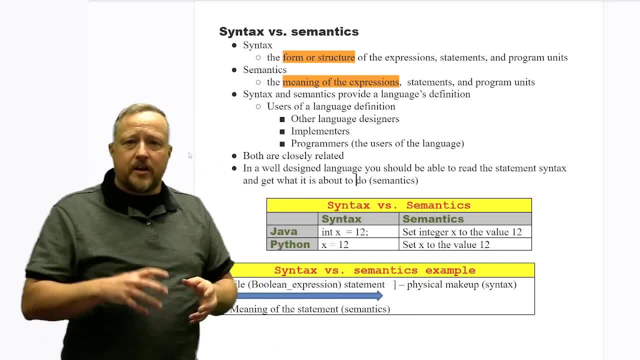 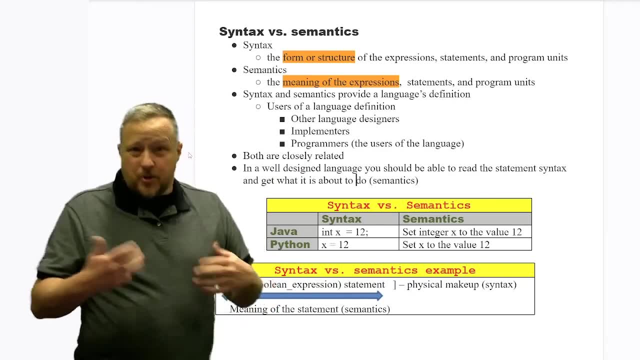 and the language definition. to try to keep things short, sweet to the point, making sure that syntax-wise and semantics, it's well, frankly, attractive Because you want to be able to use it. So both are very, very much related. So, syntax-wise, when we look at Java and Python, 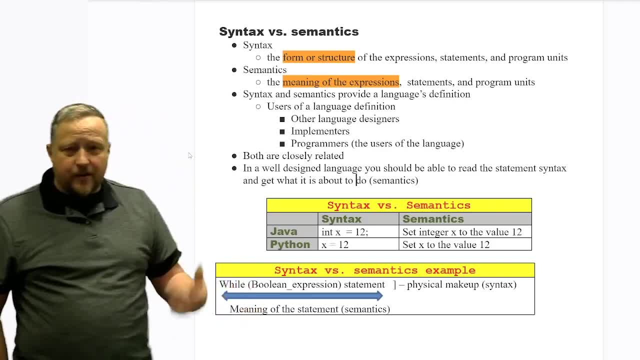 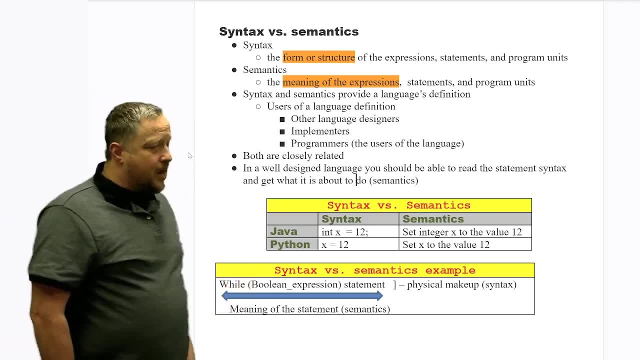 we know the syntax between the two when it sets to setting a variable to 12.. But what's the meaning behind it? the semantics behind it can be very different, Especially when it comes to Python, we don't declare data types, whereas Java man, we're really locked into having x be an integer That makes a difference. So that's the